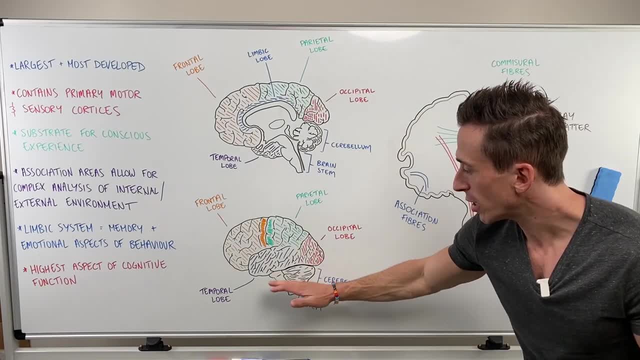 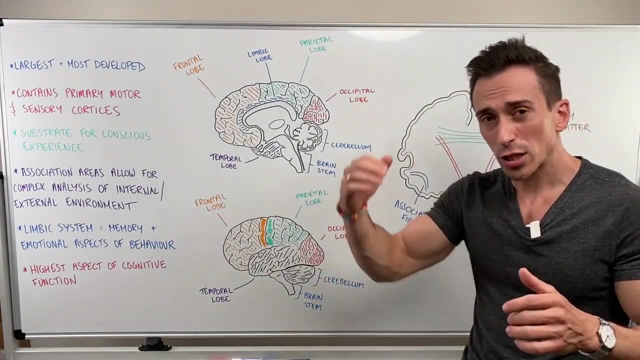 and towards the back and the brain stem underneath, which sits just above the spinal cord. Today we're talking about the largest part of the brain, which is the cerebrum, which has a fissure or segmentation down the middle that separates it into two hemispheres: a left, 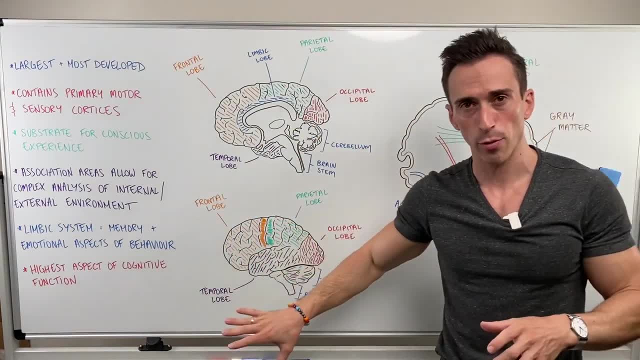 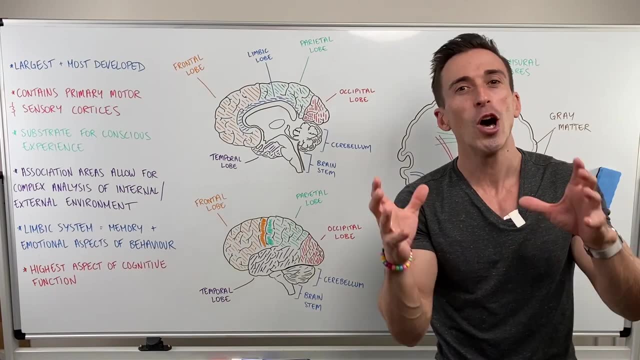 hemisphere and a right hemisphere, So it's the largest part of the brain, but it's also the most developed part of the brain. Now, what do I mean by developed? Well, let's take a look at some of the functions of the cerebrum, First of which is that the cerebral hemispheres. 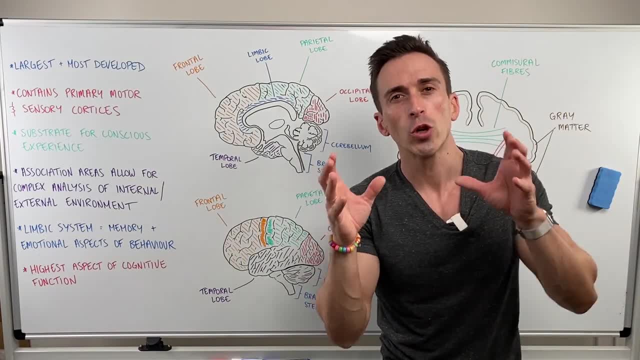 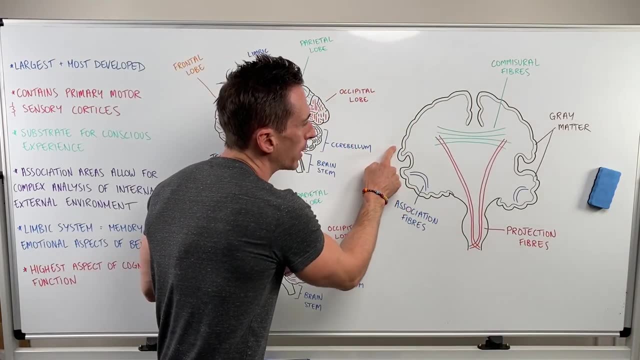 contain the primary motor and sensory cortices. Now, when I say cortices, I'm referring to the cortex, and the cortex is simply the outer one to five millimeters of the cerebrum. It contains grey matter. Remember, when we look at a neuron, you're 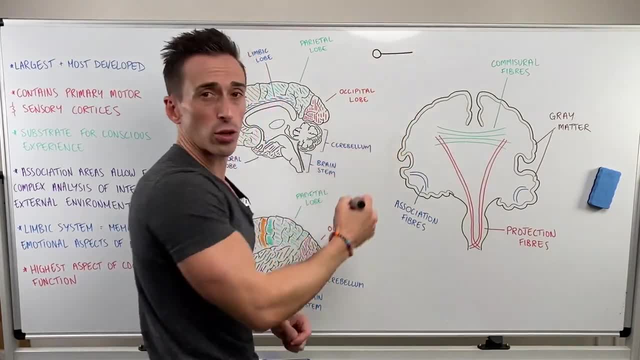 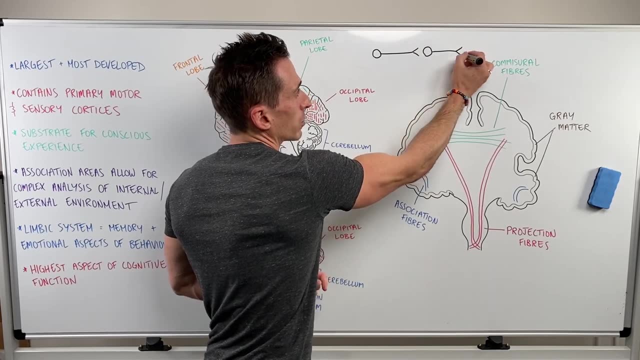 going to have the cell body of a neuron. you're going to have the axon of the neuron and then you're going to have the axon terminals. That axon terminal is likely going to talk to another axon or neuron. I should say, for example, So importantly, the axon is surrounded. 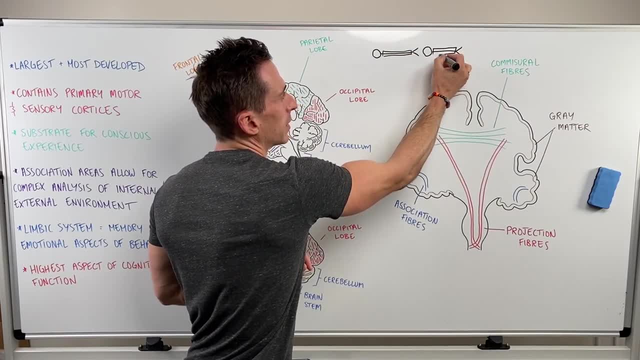 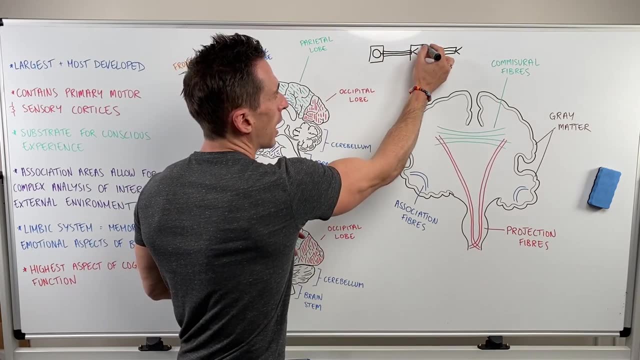 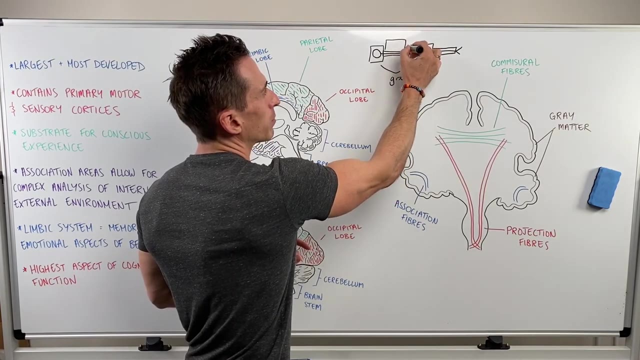 by fat- myelin and fat in this case- looks white. So when we look at grey matter, grey matter are the cell bodies and the areas of synapsing, So that's grey matter And the white matter is actually simply the axons. So that means that when you see grey matter, this is the 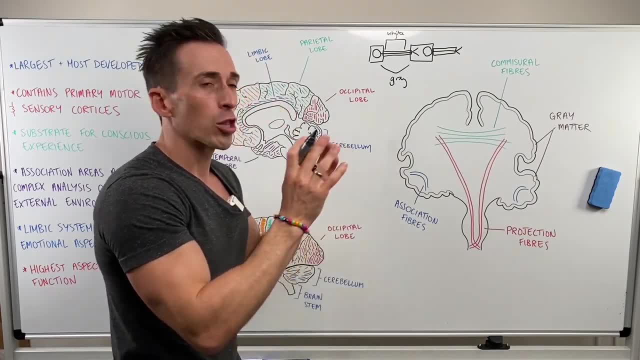 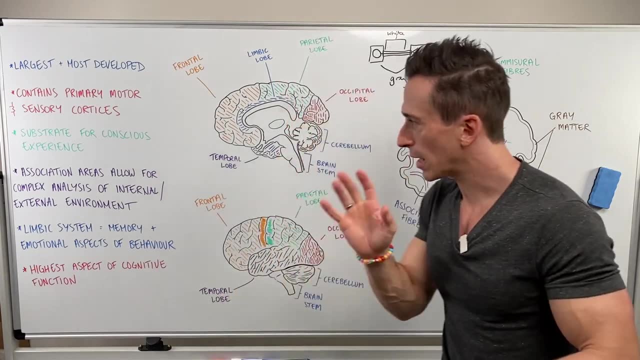 side of integration, where we make sense of information. The white matter is simply just highways. This is simply where one signal is sent to the next area. All right, Keeping that in mind, when we look at the primary motor and sensory cortices, we're going to 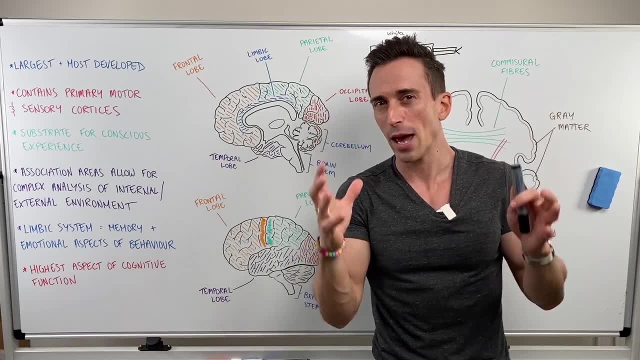 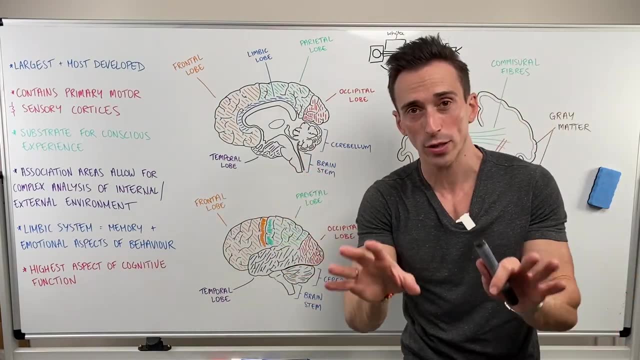 look at the primary motor and sensory cortices that sit within the cerebral hemispheres. This is the highest level of activity, For example, when we look at the motor cortex or the primary motor cortex, which actually sits in this part of the frontal lobe. this 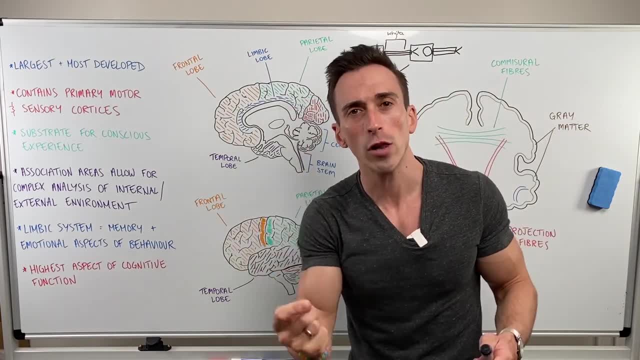 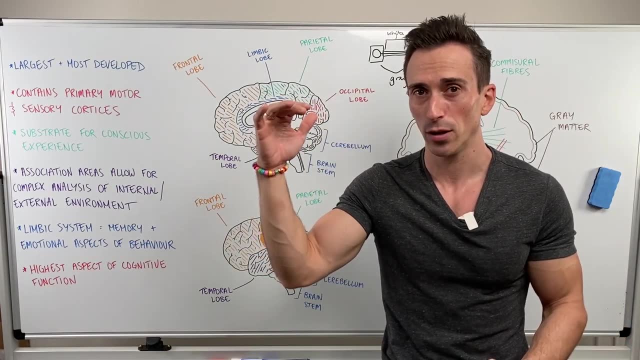 is the area where we want to initiate some sort of voluntary or conscious motor movement. If I want to begin walking, this is where it begins, So that's why it's the highest level in which motor activity will function. When we look at the 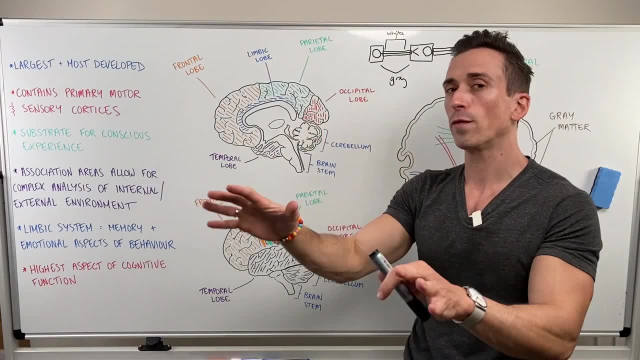 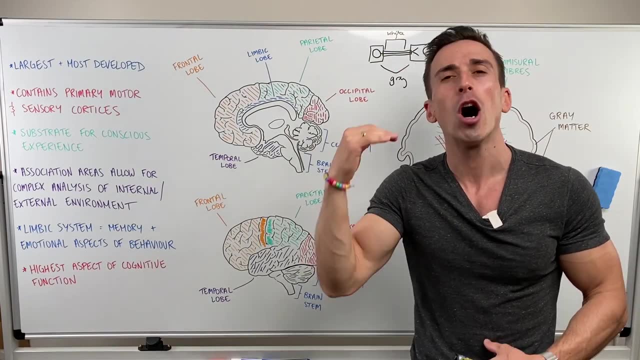 sensory cortex. this is where information coming from the external environment or the internal environment is coming up for us to be consciously aware of it. Again, it's the highest level of integration of sensory information. This is where we become aware. So think about. 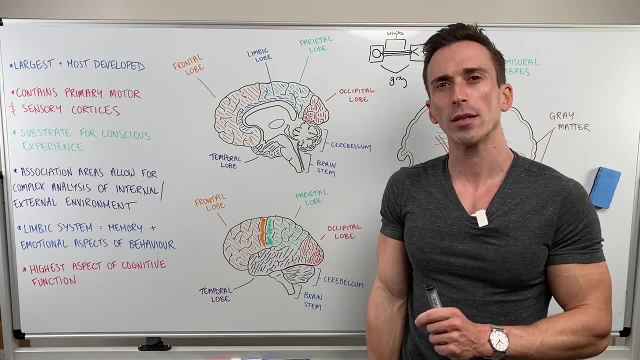 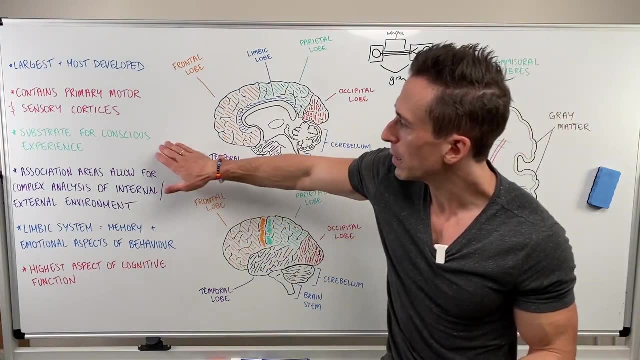 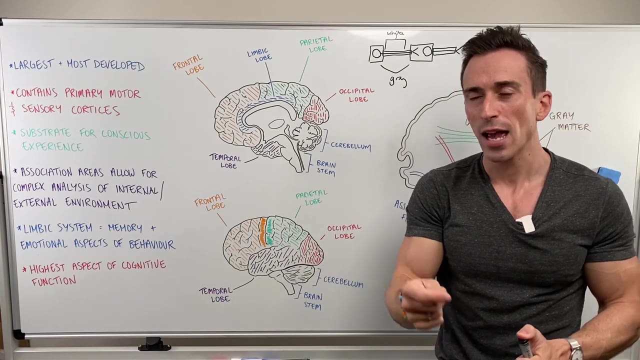 if you had your hand in your pocket. when you feel something in your pocket, this is going to the sensory cortex. All right Now, in addition to that- I'm going to skip this part- here We've got association areas, The association areas. they help the primary motor and sensory cortices. 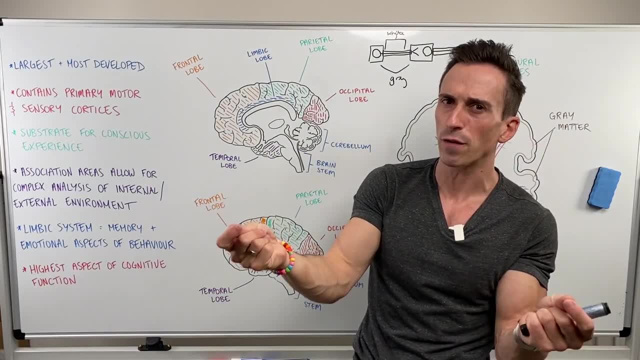 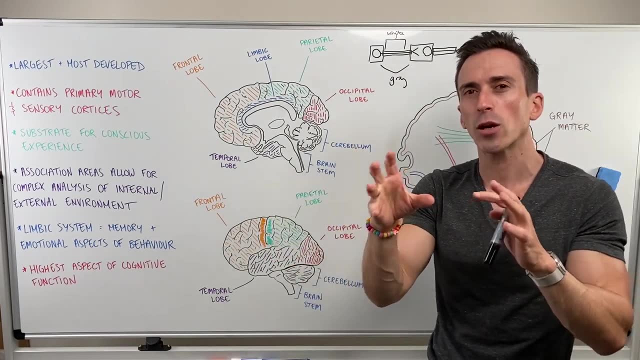 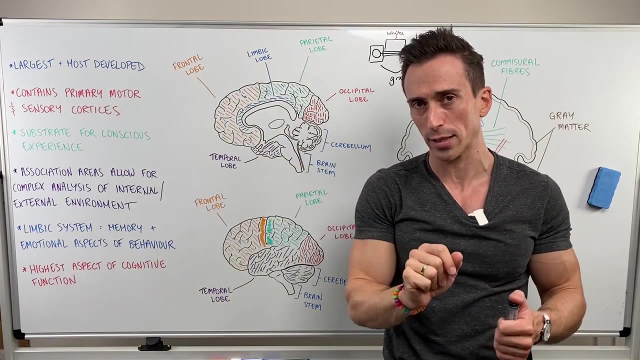 By associating previous information and current information. it's comparing and contrasting what it already knows so that you now have more information. It's basically a way to analyze complex information. So, first of all, the association areas for the motor cortex. So I said you're going to have the motor cortex here. I want to initiate walking, for example. 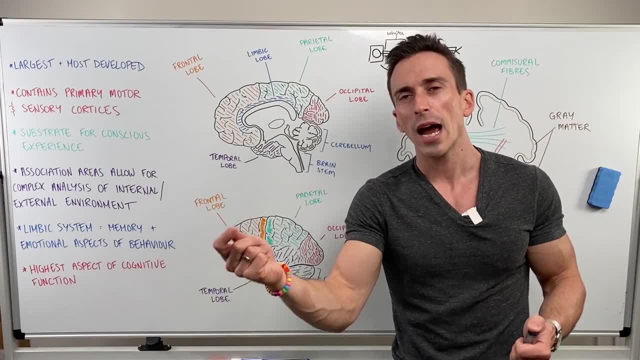 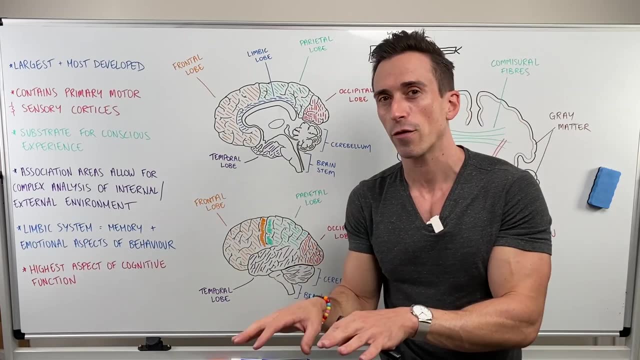 sitting there at the primary motor cortex, But the association areas allow for you to sequence and plan more complex tasks. So if I wanted to go play the piano, for example, or juggle some balls, this is where we have the association areas come into play. for the 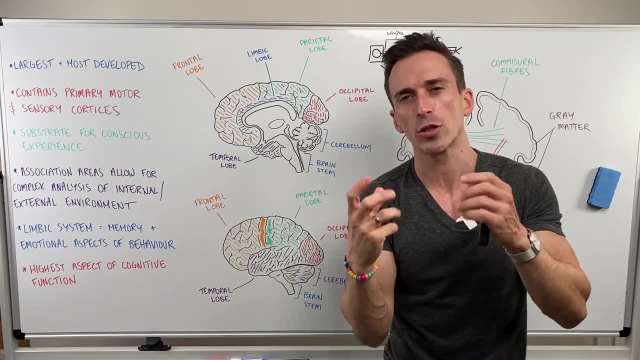 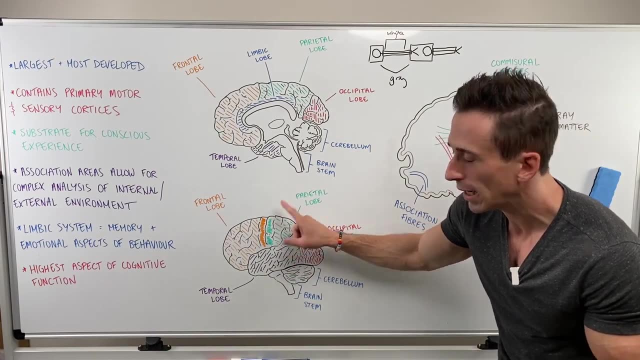 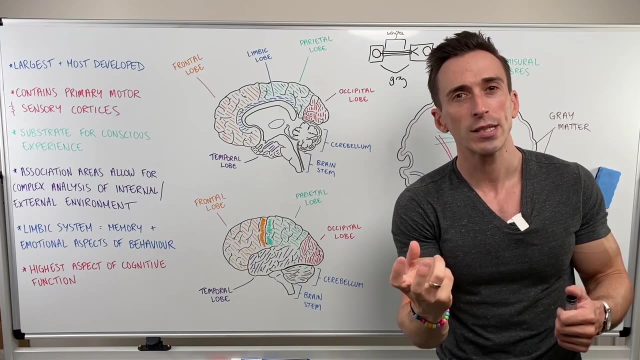 motor cortex. It allows for us to plan and sequence complex movements. When we look at the sensory cortex, which I didn't say sits within that parietal lobe, here the association cortices help you understand what piece of sensory information you are receiving. 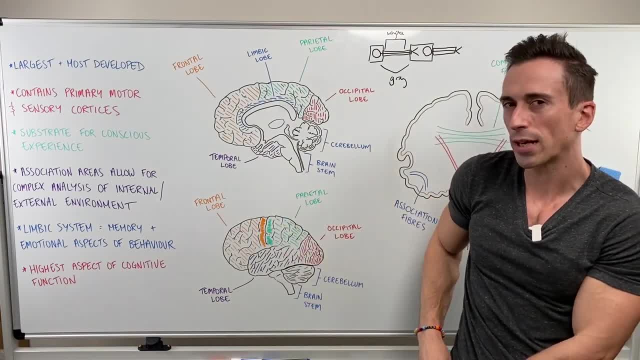 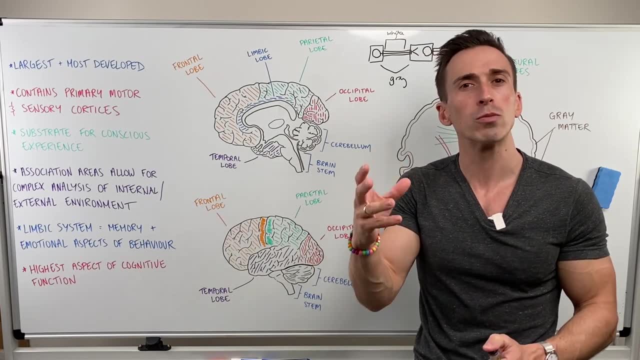 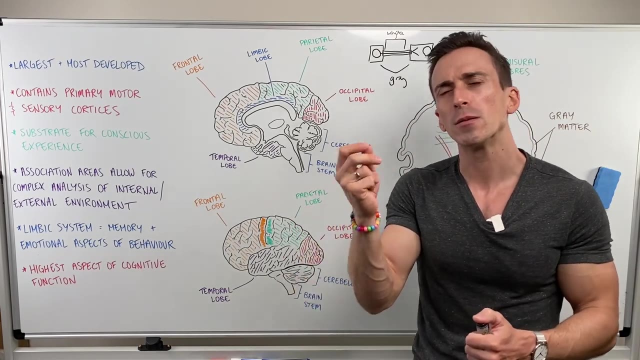 So I said before that primary sensory cortex. there you put your hand in your pocket and you feel something. What the association cortex does is it analyzes whether it's smooth or rough, whether it may be hot or cold. Have I felt it before? What might this be from previous experience? 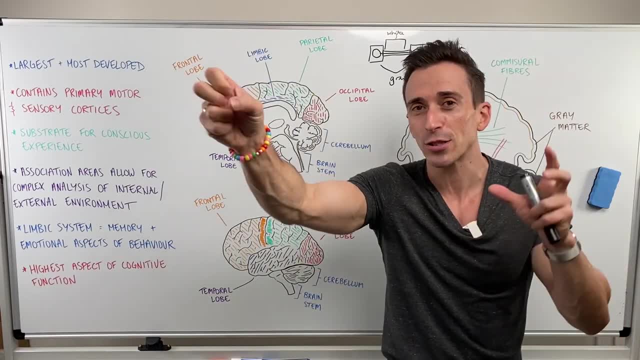 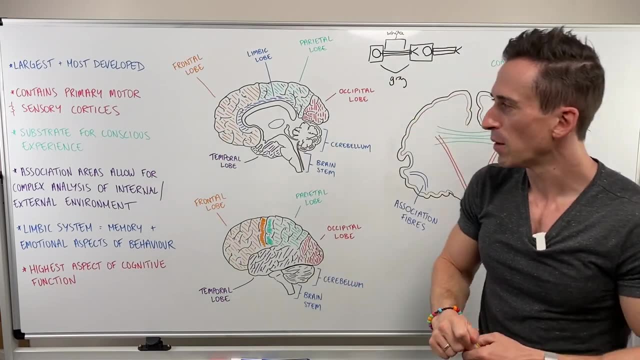 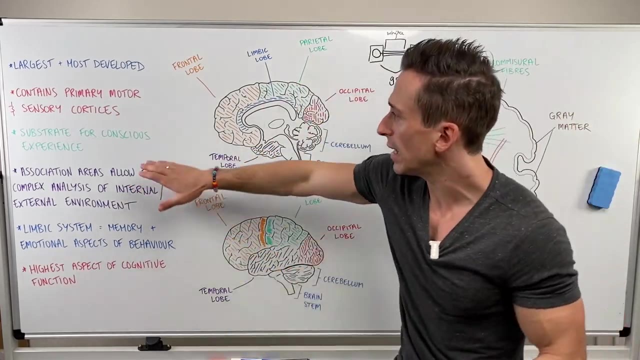 So it's an association cortex because it's bringing associations from previous experience, Throwing it to that of the primary somatosensory cortex. So these are these association areas, all part of the cerebral cortex. The cerebral hemisphere is the substrate for conscious. 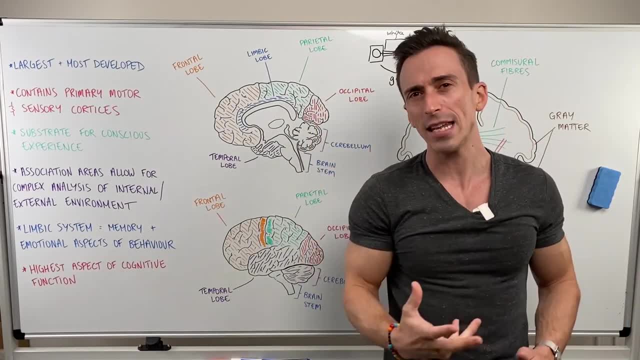 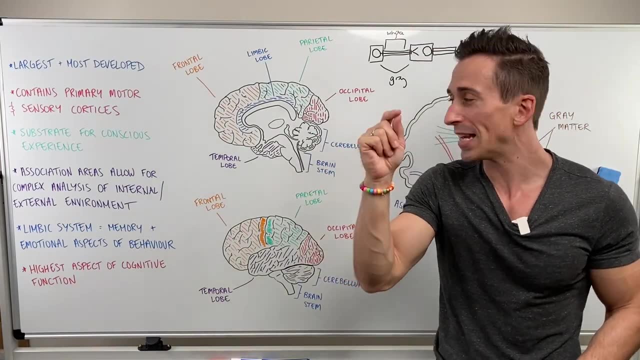 experience. When we become consciously aware of anything, it's because it's gone to the cortex of the cerebral hemispheres. So if you want to be consciously aware, it needs to get to those one to five centimeter thick millimeter I should say. 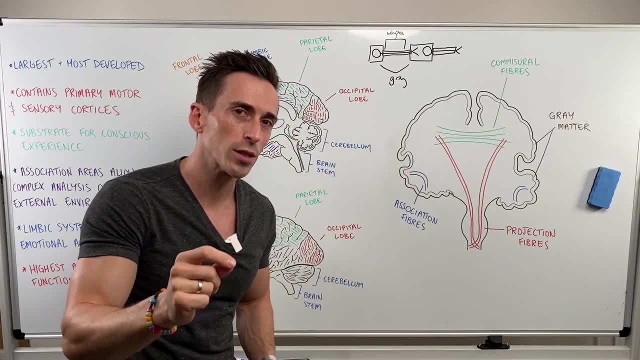 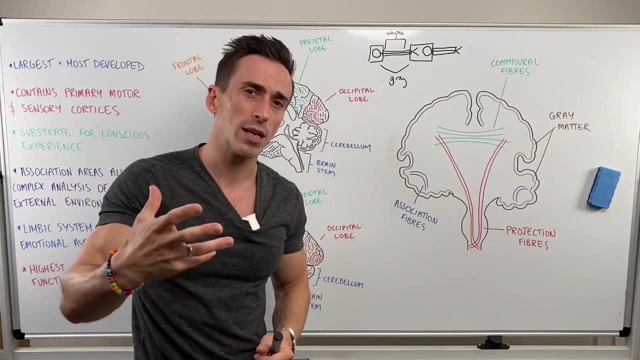 layer of the cerebral hemispheres. If you want to be consciously aware, this is where consciousness is going to arise, where you become aware of experience. More deeper areas of the brain may receive sensory information, but you will not become aware of it occurring, Or it may make a 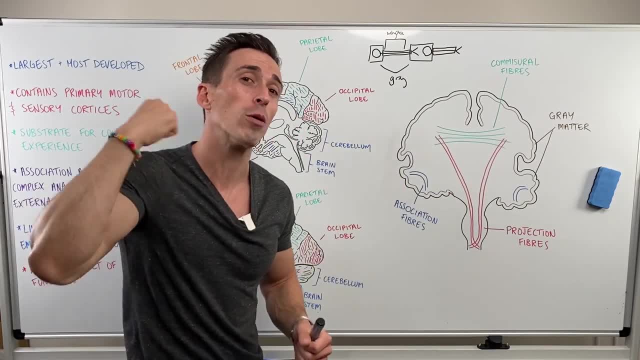 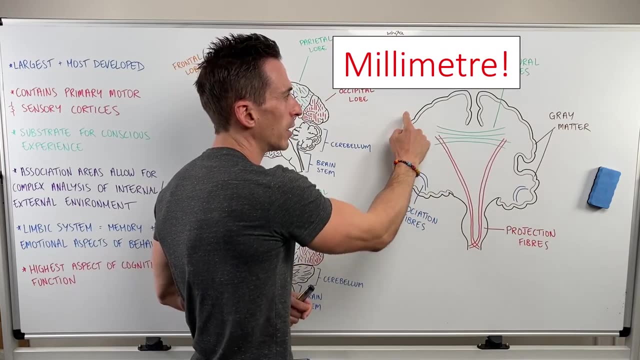 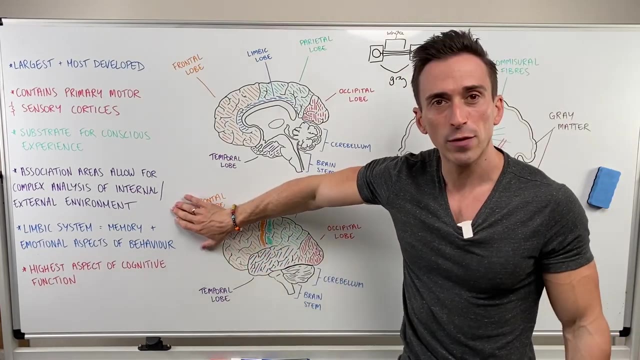 decision about conscious, may make a decision about motor movement, but you're not going to be consciously aware of that. For conscious awareness, it must get to that one to five centimeter external layer that we call the cortex of our cerebral hemisphere. The cerebral hemispheres also contain the limbic system. Now, the limbic system is important for 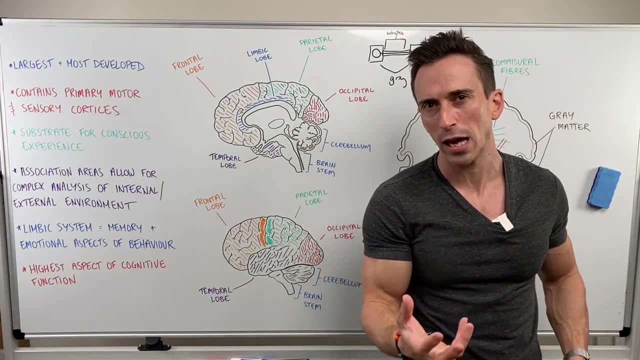 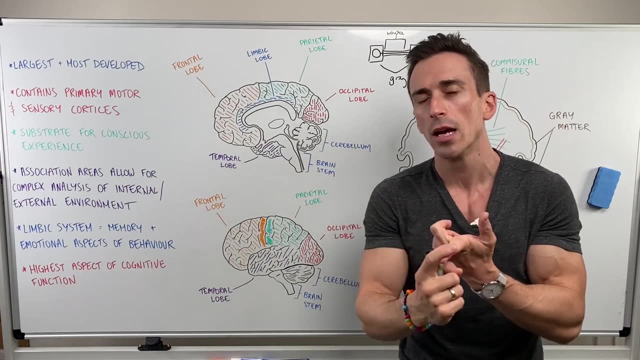 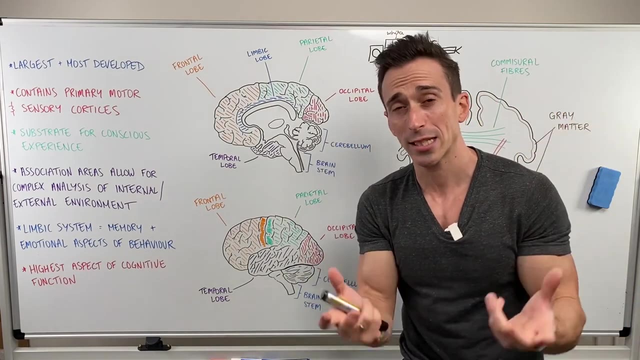 memory and emotional aspects of behavior. So think of emotional aspects of things that you do. So the emotional aspects of feeding, the emotional aspects of relationships, the emotional aspects of reproduction, the emotional aspects of fight or flight. This is the limbic system and you can see. 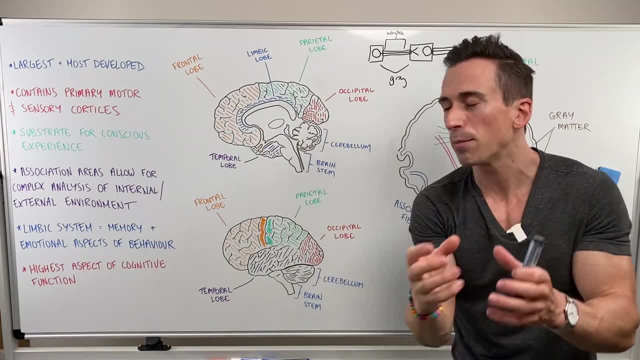 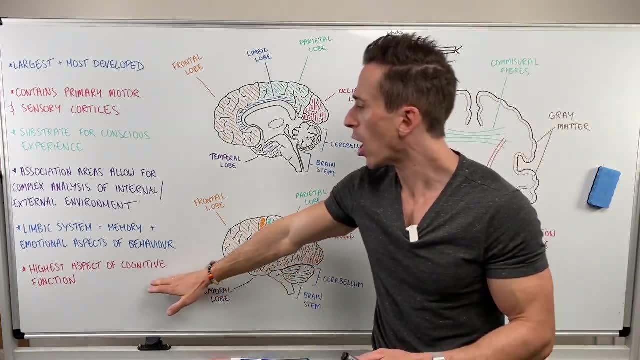 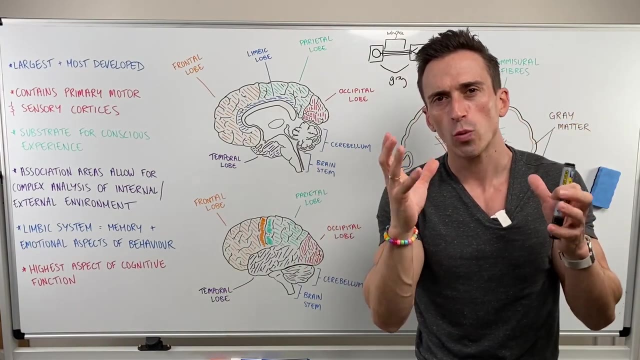 part of the limbic lobe. sitting here There's deeper limbic structures as well, right near the thalamus that you can see here. So we've got the limbic system. It's also the highest aspect of cognitive function. The cerebral hemisphere is the highest aspect of cognitive function. So when we look at cognitive 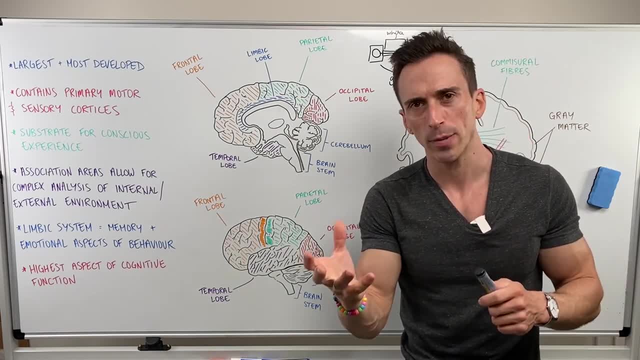 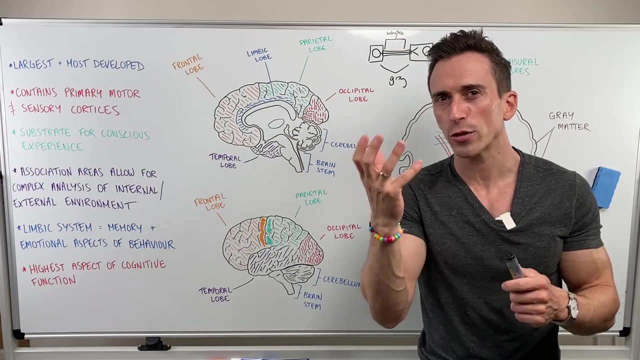 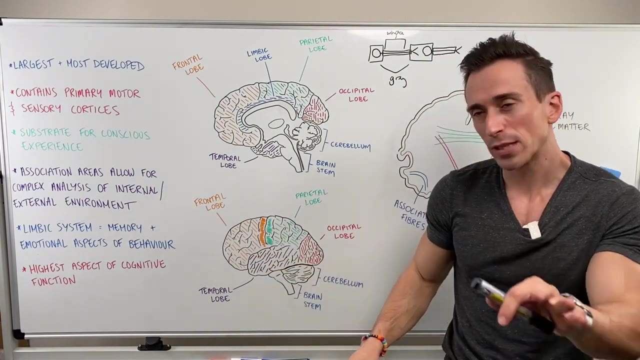 function. we're thinking about planning, judgment, emotion, making sense, being reasonable, making sure that your behavior is appropriate for the scenario in which you're in. Most of this sits within the frontal lobe, specifically an area called the prefrontal. 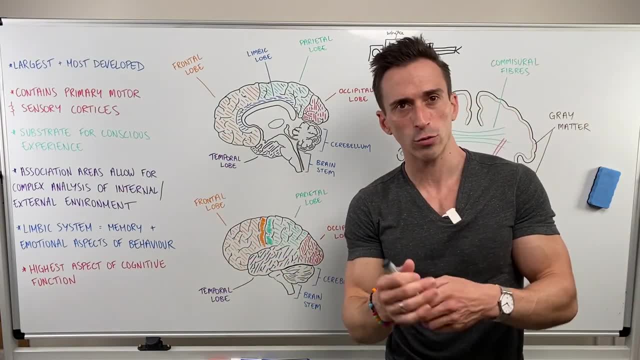 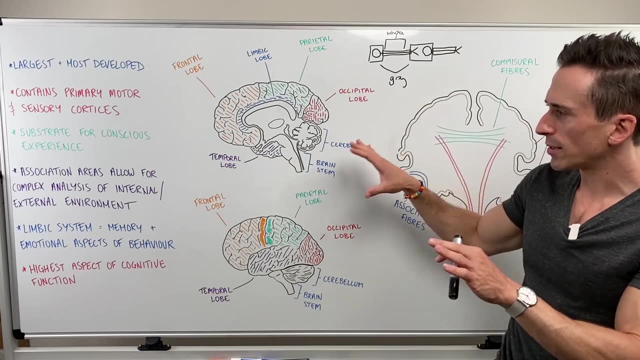 cortex. If that area is damaged, we have issues when it comes to behavior and planning and things like that. All right, So highest aspect of cognitive function. Now, like I said, when we take the cerebrum, it's going to have the one to five millimeter layer and then there's going to 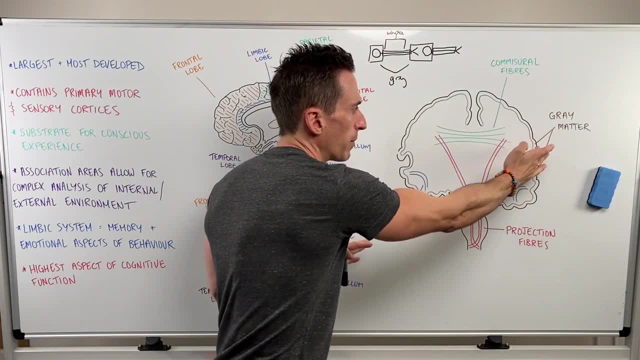 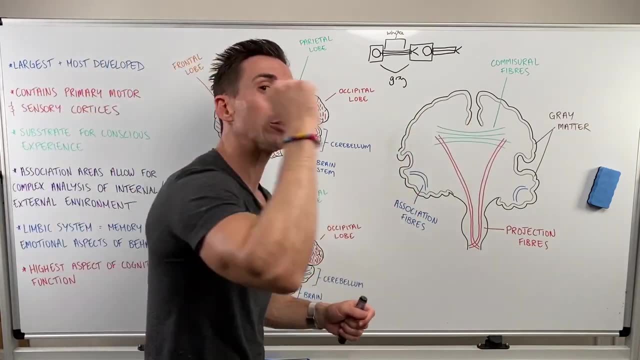 be some deeper structures. The one to five millimeter layer, like I said, is the gray matter. That's the side of integration and making sense and consciousness, Dr Justin Marchegiani. But we've got deeper layers of the cerebrum where we project information. These are the highways. 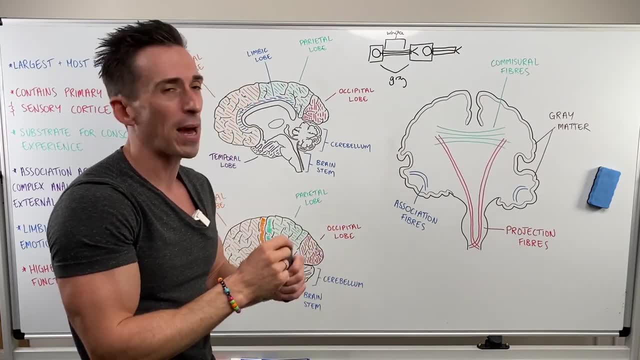 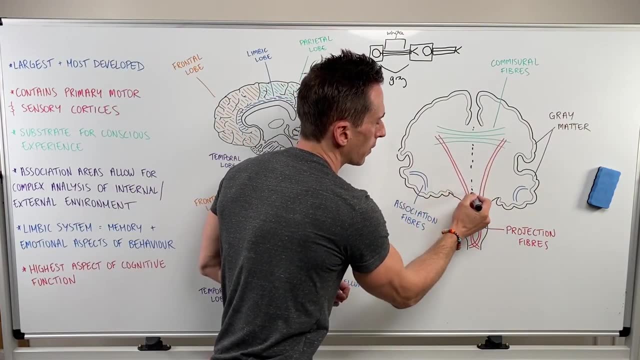 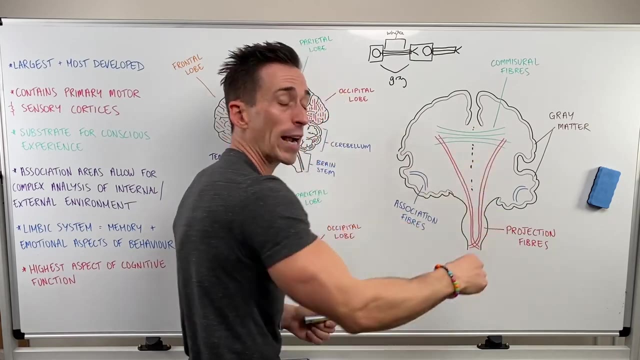 These are the axons, This is the white matter. All right, Now you can send information from one side of one, from this one cerebral hemisphere to the other, And if you do this, you're sending it through white matter, tracks or fibers. They're called commisural fibers. They are predominantly 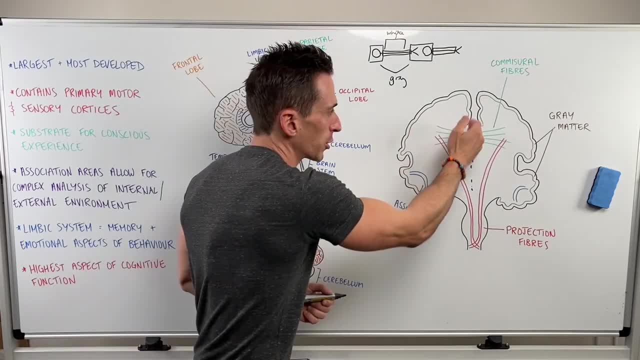 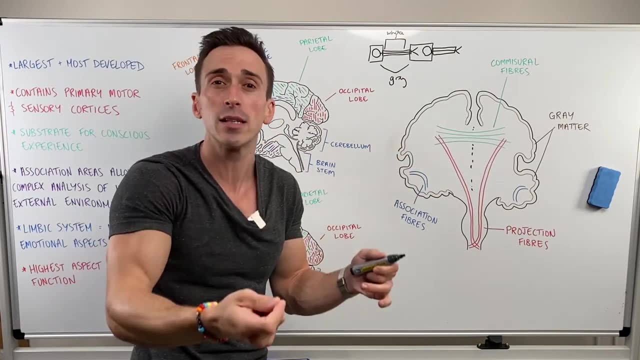 going to be through what we call the corpus callosum. That's the connection, Dr Stephen Look-on-Mitchell. Some people had a corpus callosotomy. Otomy means to cut. It separates those hemispheres. These individuals had very severe cases of epilepsy. And epilepsy is this misfiring of? 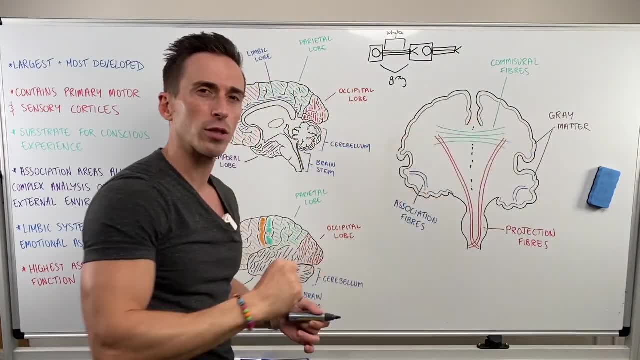 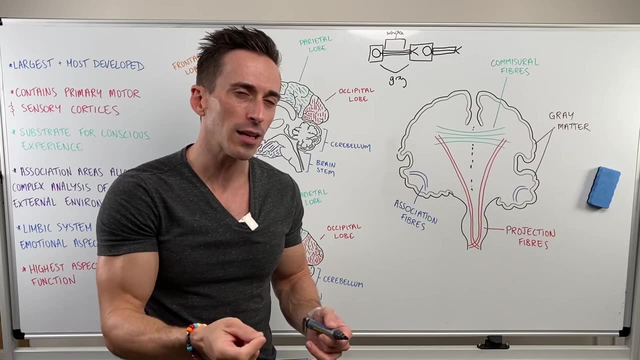 neurons. If you cut it, it stops it from spreading across the two hemispheres and help mitigate the severity of the epilepsy, But it also separated the hemispheres anatomically And if you have a look at the split brain experiment studies, you'll find some very interesting things when it comes to 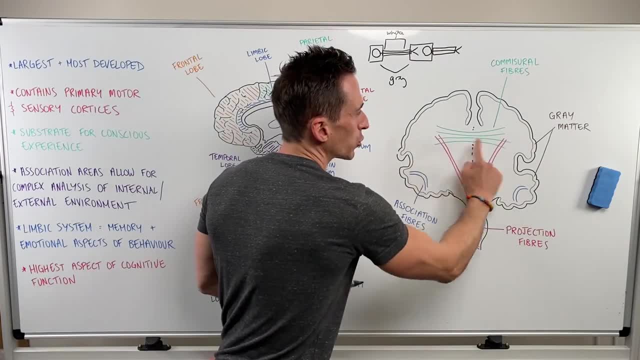 splitting the conical hemispheres. Dr Justin Marchegiani, What is the difference between this and the corpus callosum? Dr Stephen Look-on-Mitchell, consciousness of the brain. So we've got the commisural fibers from one hemisphere to the. 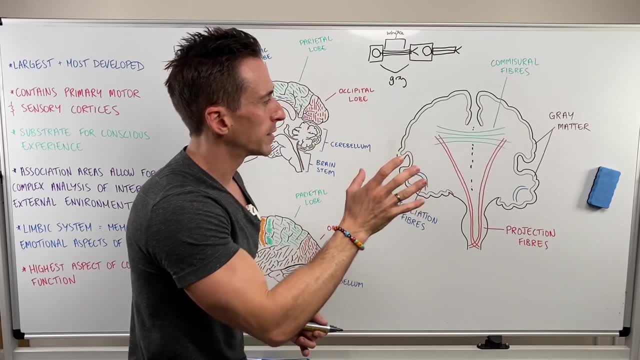 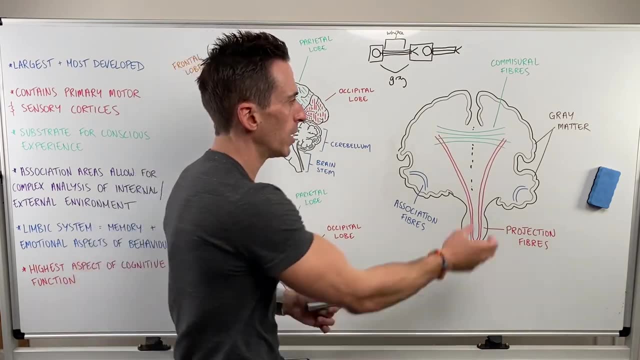 other. We've also got projection fibers. These fibers take it from more superficial areas of the brain to deeper aspects of the brain, brainstem and spinal cord. These are going to be projection fibers. You can see that they're going to cross over to the other side because the right hemisphere 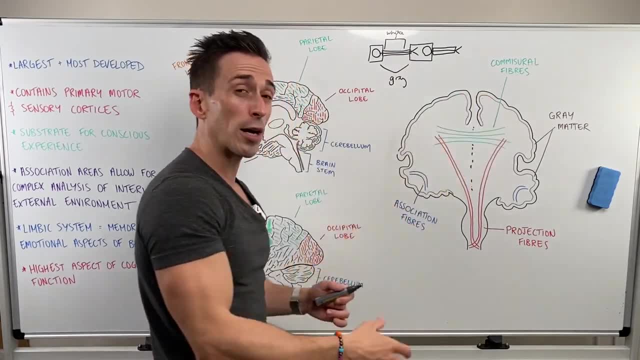 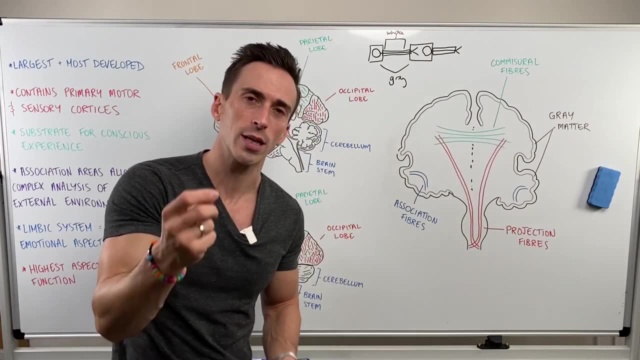 controls the left-hand side of the body. left hemisphere controls the right or the right side of the body, sends information to the left hemisphere and vice versa, which means these projection fibers must cross at some point. Usually they're going to cross at around about. 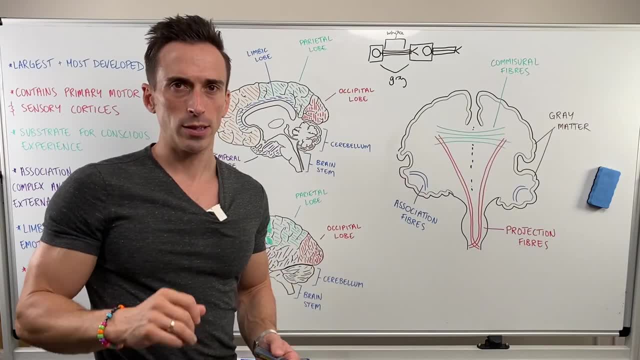 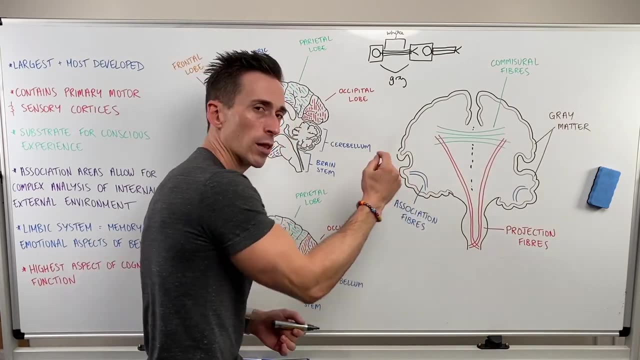 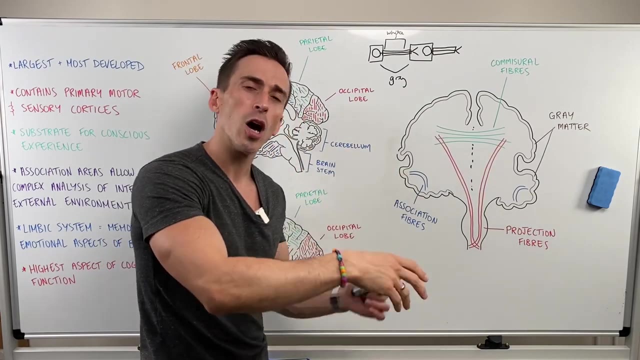 the medullary region Association fibers. I spoke about association areas. Association fibers allow for one part of the cortex to speak to another part of the cortex so that we can make more sense of what's happening in the situation. If I want to sequence a motor task, I need these association 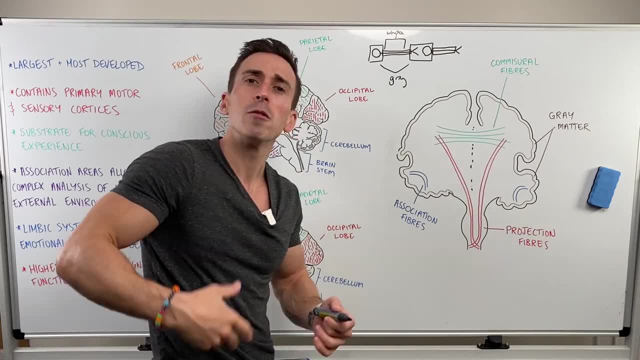 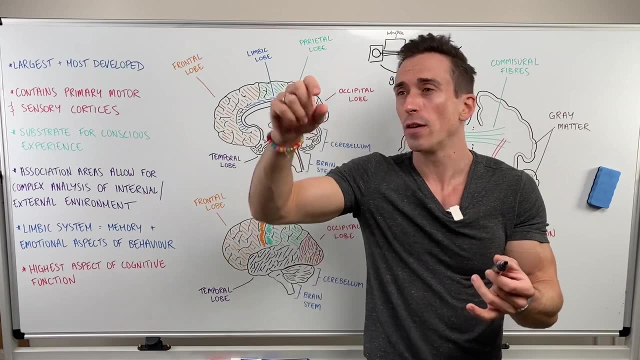 fibers. If I want to make sense of what I'm feeling, I need these association fibers. If I want to make sense of what I'm feeling in my pocket, again, we need these association fibers. So when we look at the cerebral hemispheres, it's made up of cerebral cortex one to five. 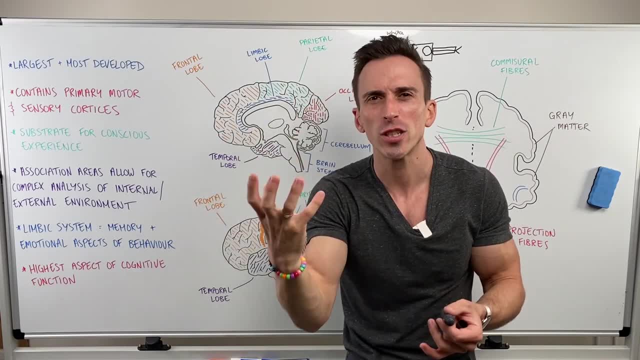 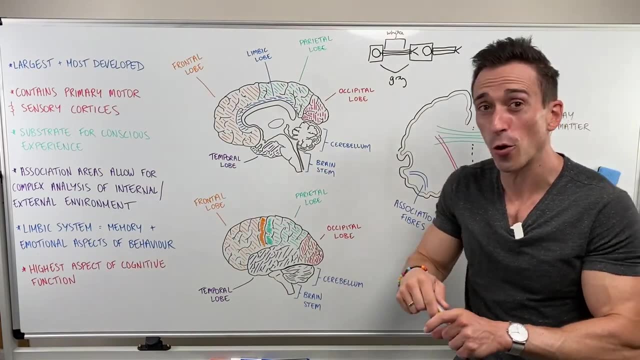 millimeter layer. This is the site of what is it? Consciousness, experience, integration. It's made up of lobes and these lobes, which we should probably look at before we finish, I'm going to focus more attention on those lobes in future videos. These lobes are made up of the frontal. 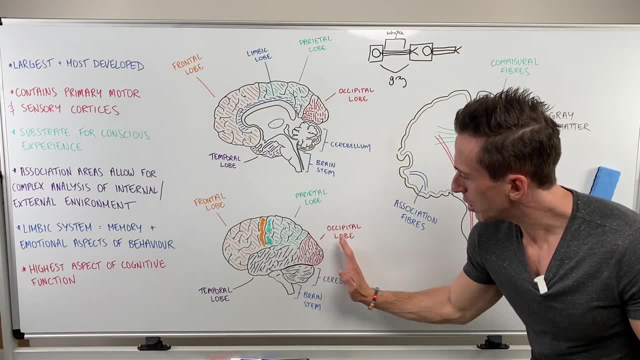 lobe, the parietal lobe, the occipital lobe and the parietal lobe At the back, the temporal lobe near the temple, And we've also got an insular lobe, If I were to. 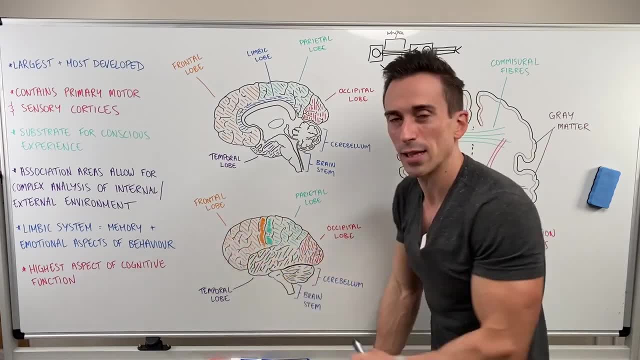 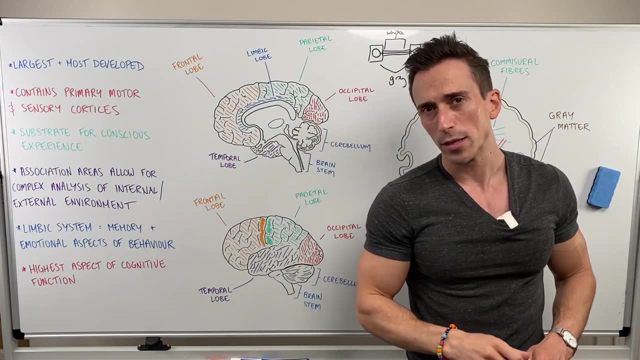 sort of pull that temporal lobe away from the frontal. you could see the insular underneath. I'm going to do videos on each of these lobes more specifically. But final point is that when we look at the superficial or surface anatomy of the brain, you're going to find that there's 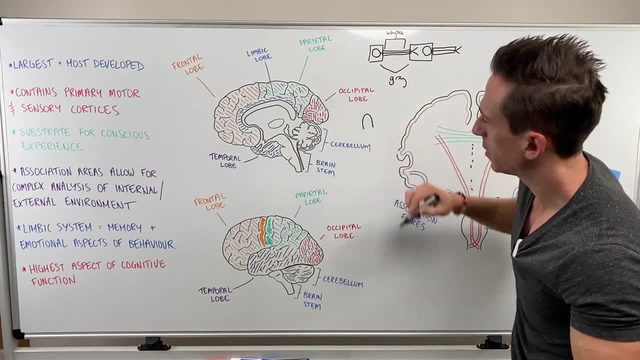 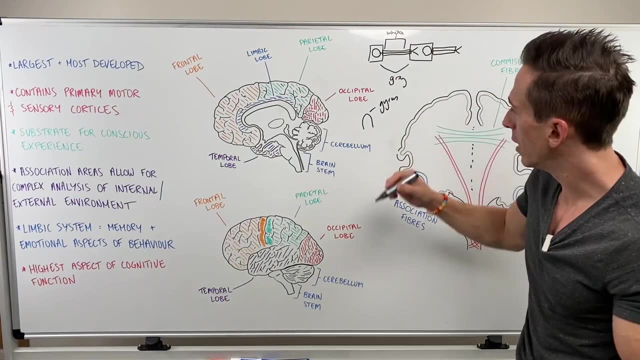 areas which have a bump up and a dip down. Now the bump up is known as a gyrus. That's singular. If it's plural, it's gyri. The dip down is known as a sulcus. Again, that's singular A. 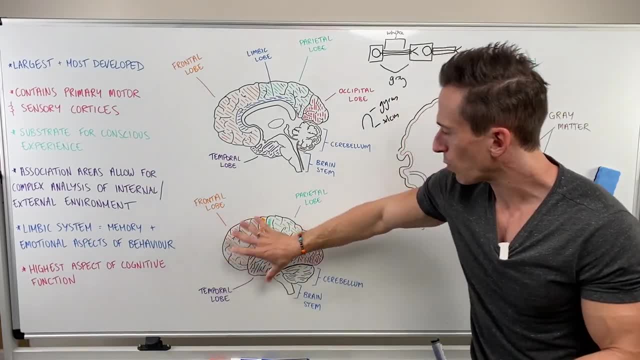 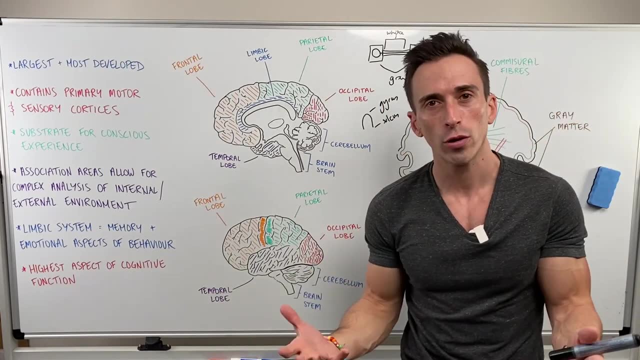 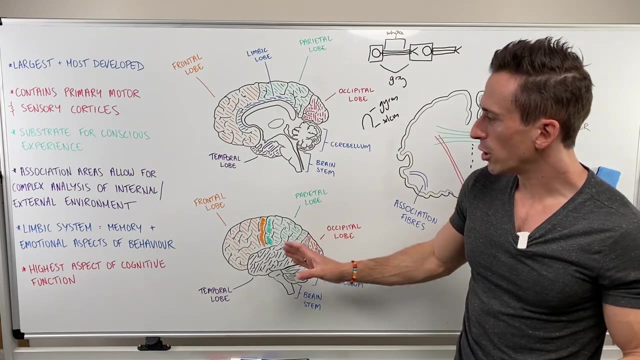 sulci is plural, And this is what gives the brain its wrinkled appearance. It just increases the surface area of the brain, which means there's more room to fit more neurons, more sites of integration, all that type of fun stuff. So a couple of points, Because I said you've got the 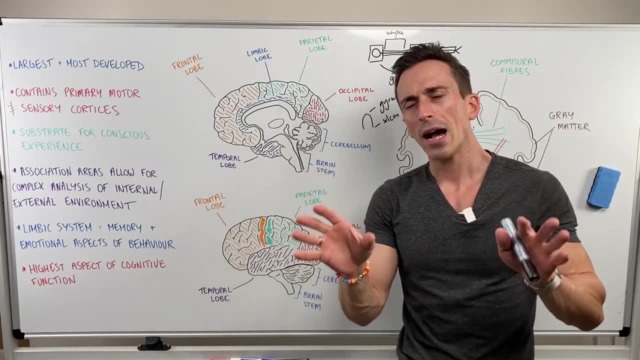 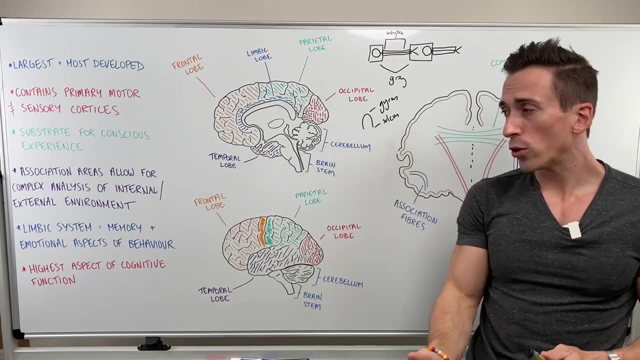 frontal lobe, the parietal lobe, the occipital lobe and the temporal lobe. how do we separate them out? How do we anatomically know where their demarcation points are? Well, we use gyri and sulci For 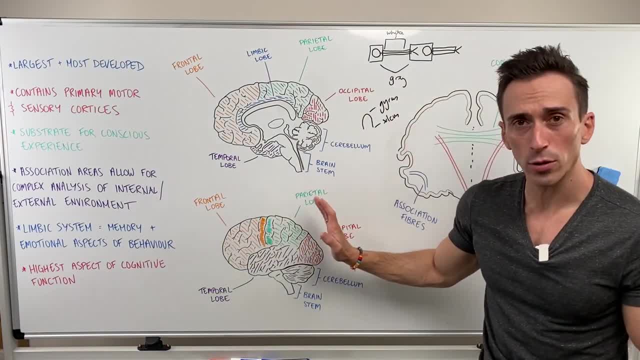 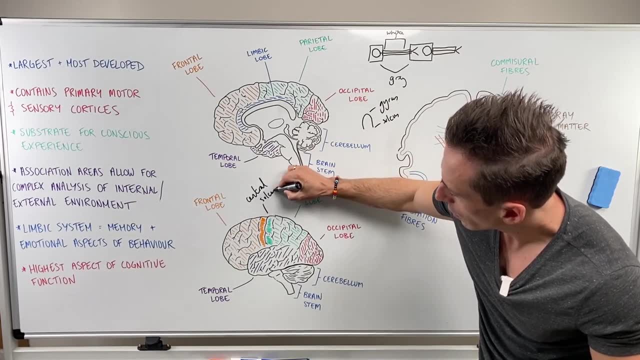 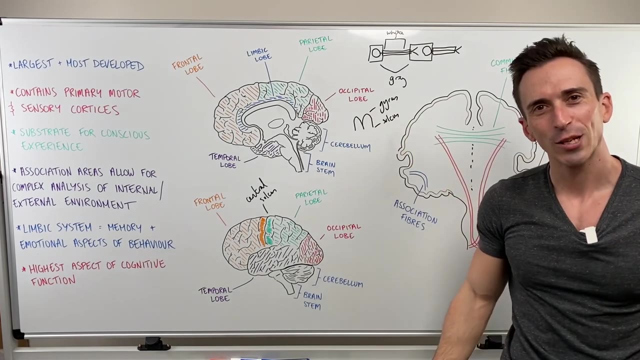 example, we separate out the frontal lobe from the parietal lobe with a sulcus called the central sulcus. Central sulcus, Now, wherever there's a sulcus in front and behind is going to be a gyrus right. So this central sulcus, we've got a gyrus in front called the pre-sulcus. 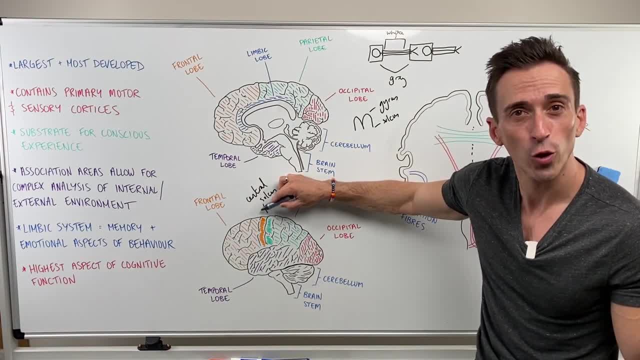 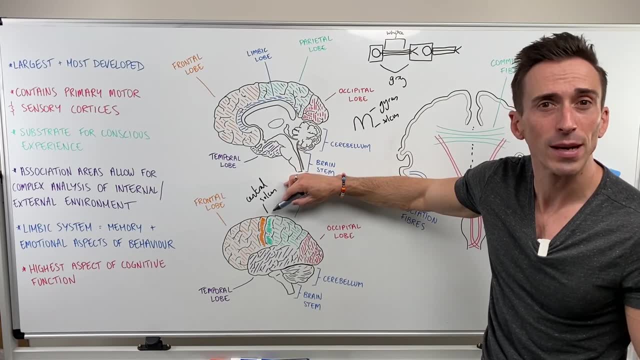 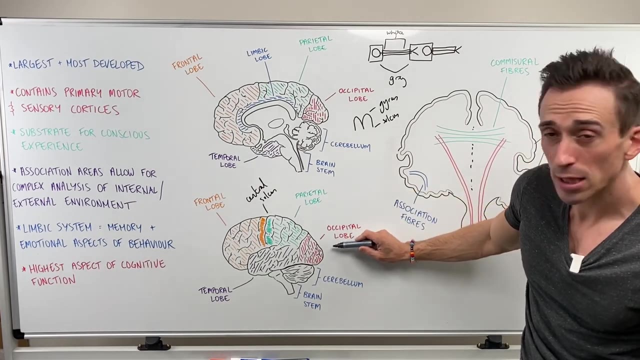 That's the central gyrus And that's that primary motor cortex. We've got a gyrus behind it And that's going to be called the post-central gyrus. That's going to be the somatosensory cortex that we spoke about as well. When we look at the parietal lobe, separated out by the occipital,